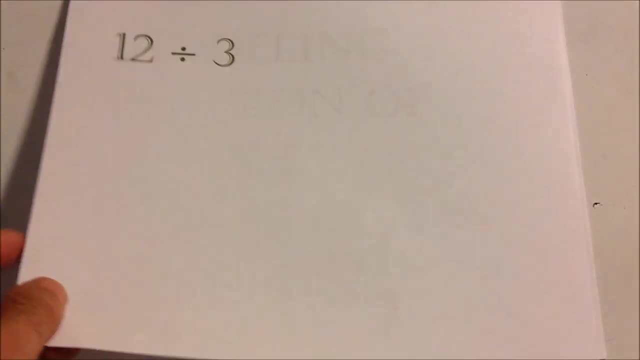 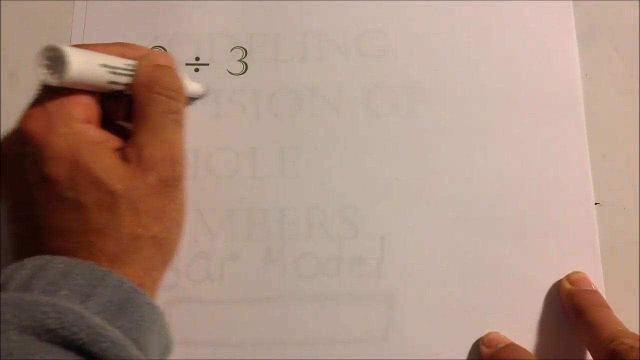 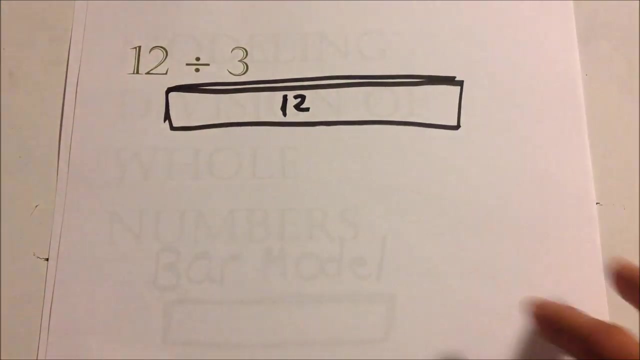 use bar models, So let's start with one. We'll do 12 divided by three. So what we have to do is we're going to make one giant bar. So here's our one giant bar, And it doesn't have to be perfect, And let's just put the number 12 in there. So that's our giant bar. Let's. 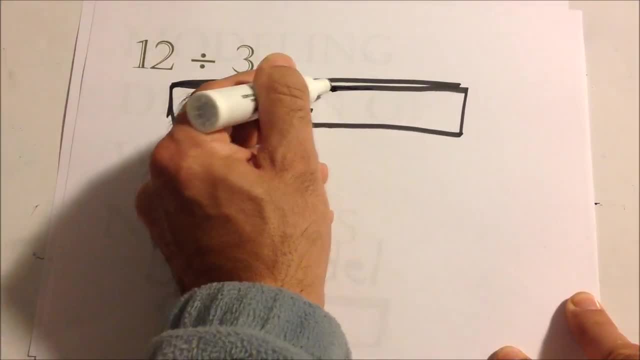 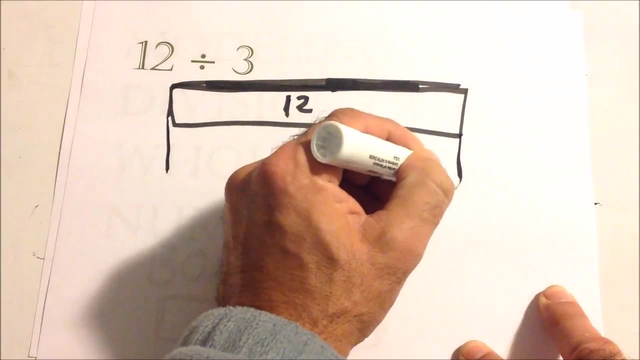 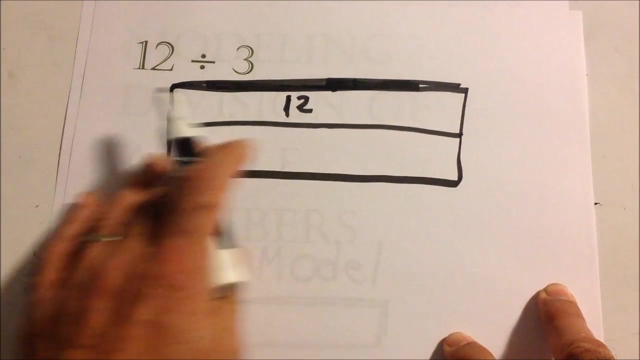 make it look a little better than that. All right, Okay. so then we want to make a bar on the bottom of it. Okay, so again, step one: we made a bar, we put the number 12. And then we put another bar on the bottom. Now we want to cut this bar three times Three. 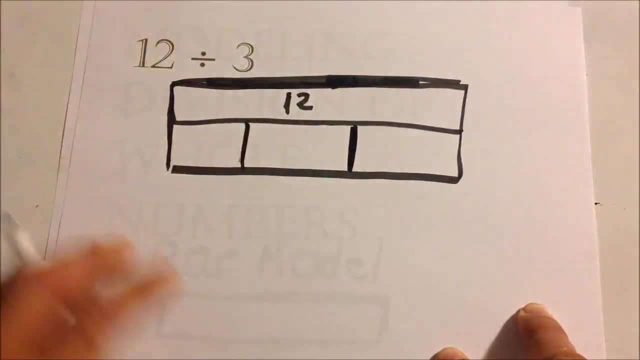 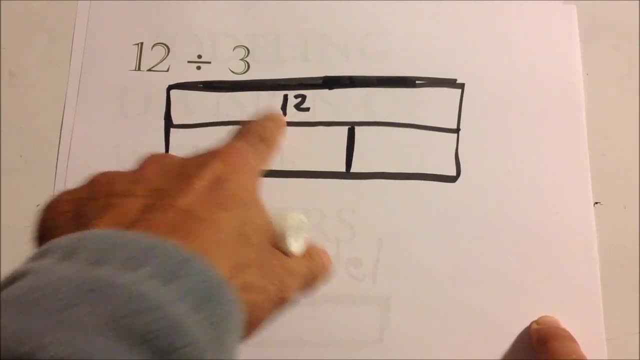 times evenly. So it looks about even. So. now we want to find out. So we have three sets here. We cut 12.. Remember this is 12 divided by three. it looks like that 12 is the dividend, Three is the divisor, Three is outside the box. Remember that, And we 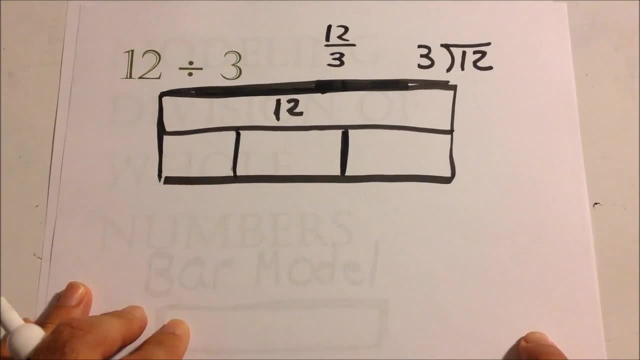 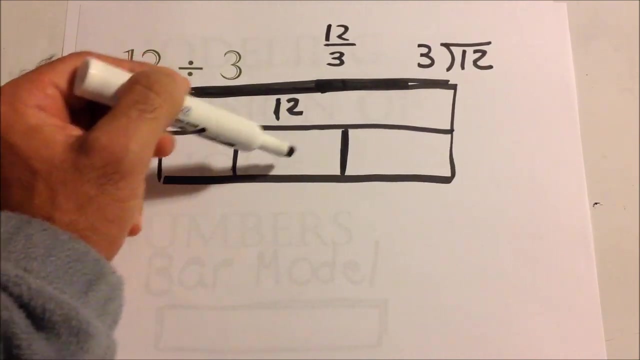 know how to do this. We've done this before in class and other videos, So here's our bar model. So how many we have these sets? we want to make each box the same. So what can we do? So what we want to do is we want to put 12 evenly into each of these boxes. So 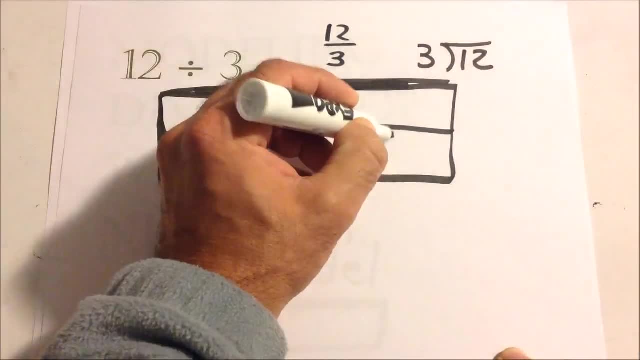 we'll do one at a time, because we have three sets. We have one, two, three, four, five, six, seven, eight, nine, 10.. One, two, three. everyone has one. One, two, three, now everybody. 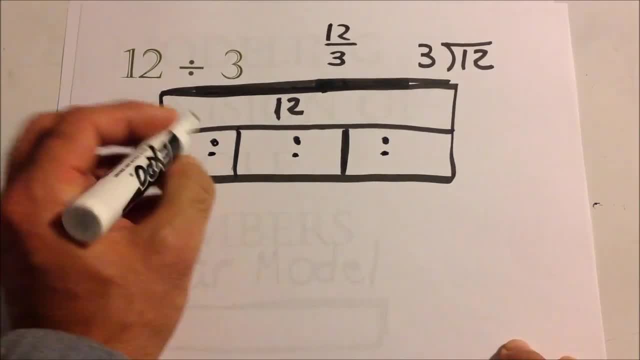 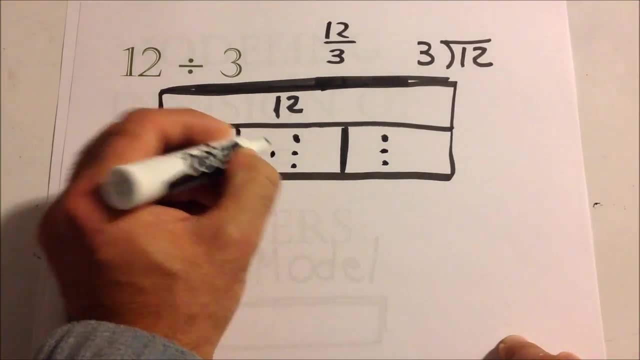 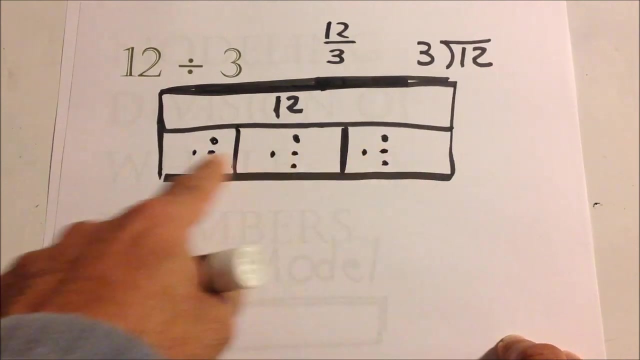 has two. is that 12? yet No, Now everybody has three, But that's not 12.. Now everybody has four, And that's 12.. So we made 12.. We cut up 12 evenly in these three boxes. So 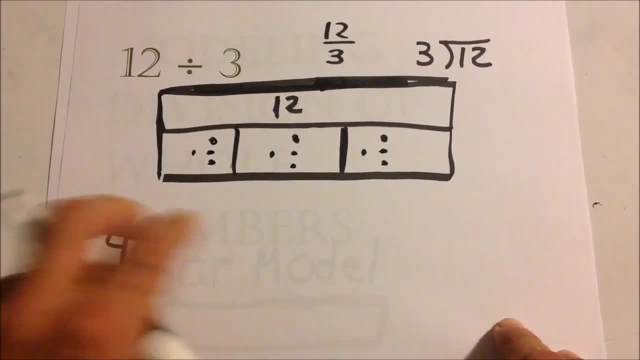 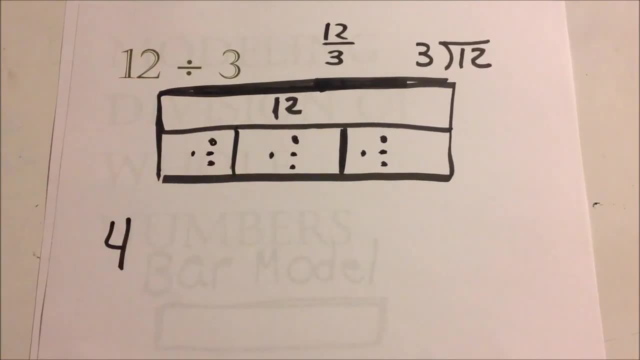 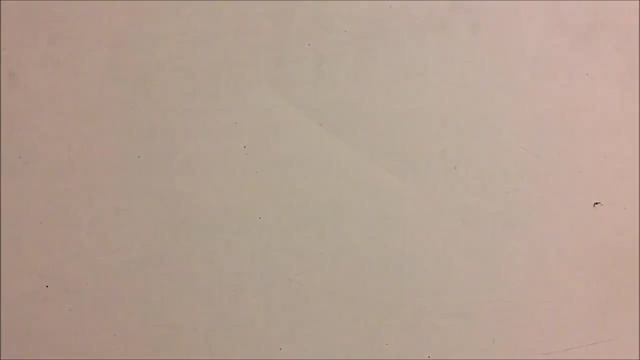 we know there are answers for Well that before. but that's how you would do. the bar model, this models this. let's see, let's see if you could do one. bring this over. what if I had? let's do 10 divided by 2, 10 divided by 2. what's the first step we should do? well, you have to make. 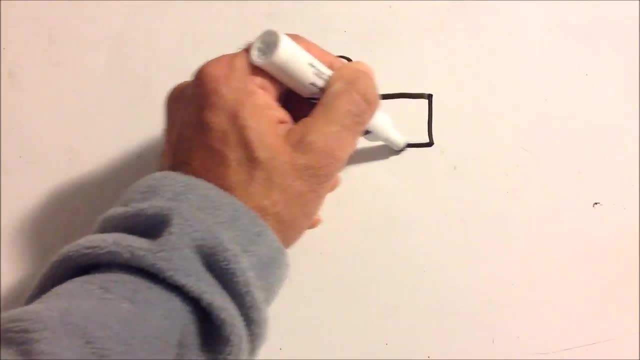 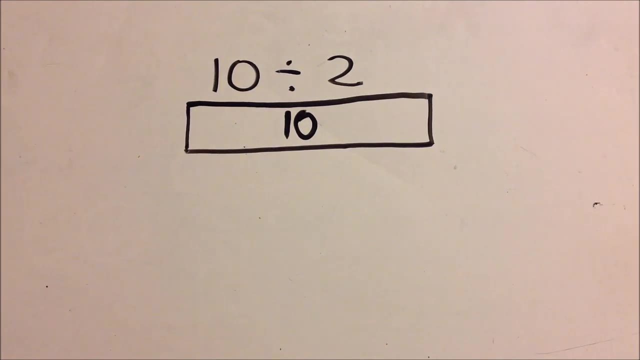 a bar. so here's our bar. and what do we put in the bar? we put the 10. good, what's the second step? right, make another bar. all right, if you want these to be chocolate bars or ice cream bars, it's your choice. right now, what is this? 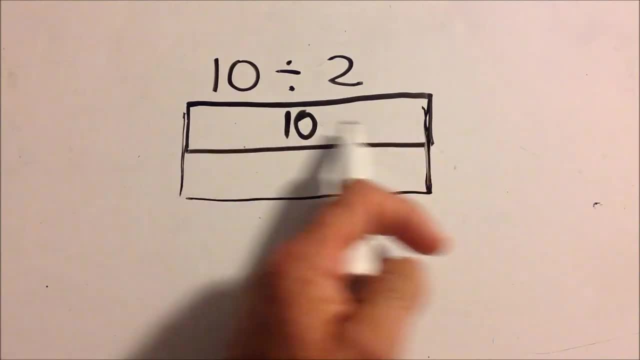 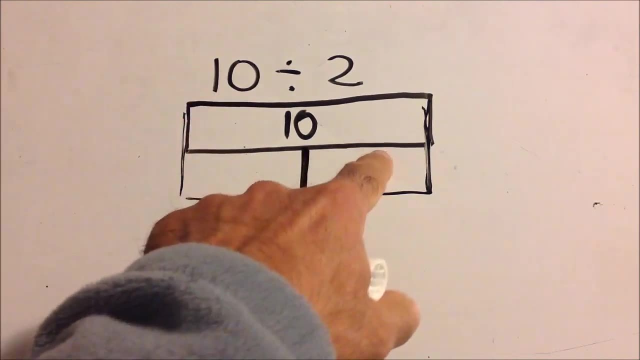 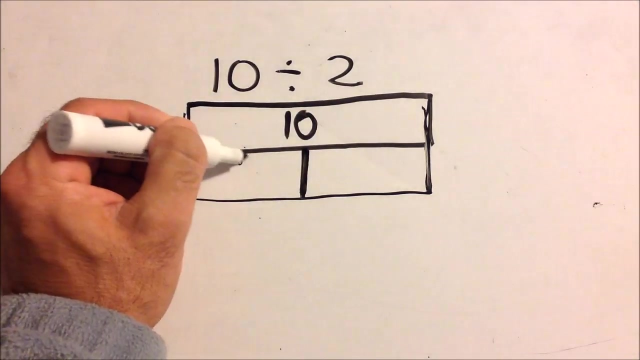 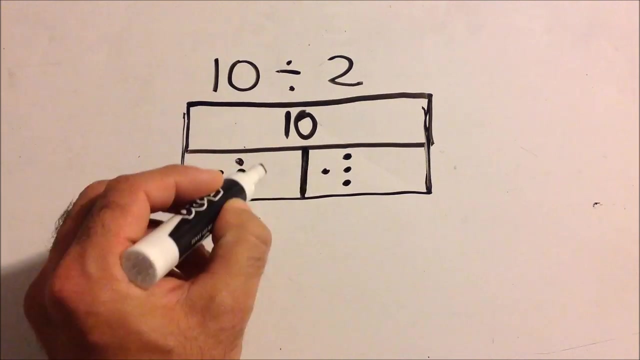 telling us to do. we want to cut this 10, this, this bar of 10. how many times two, two right in half. so now we want to fill the 10, all the 10, into these two boxes so they have the same amount. so we have 1, 2, 3, 4, 5, 6, 7, 8, 9, 10. look, we made a division. 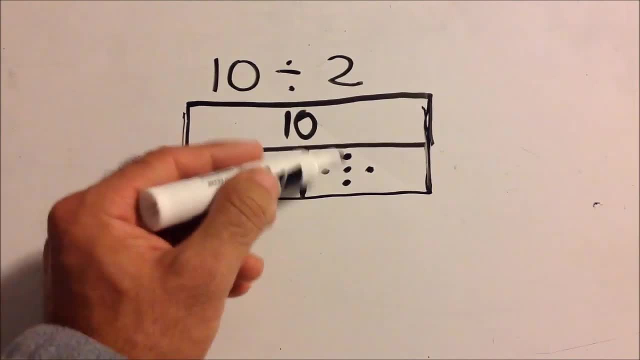 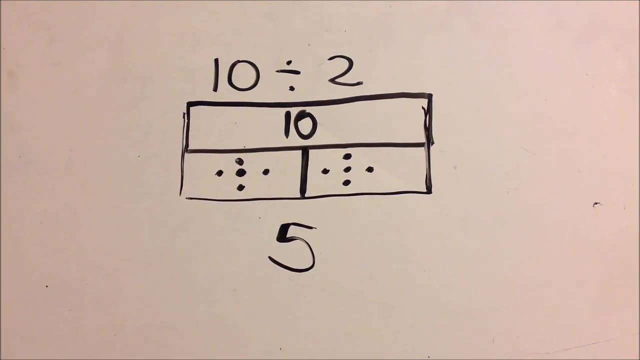 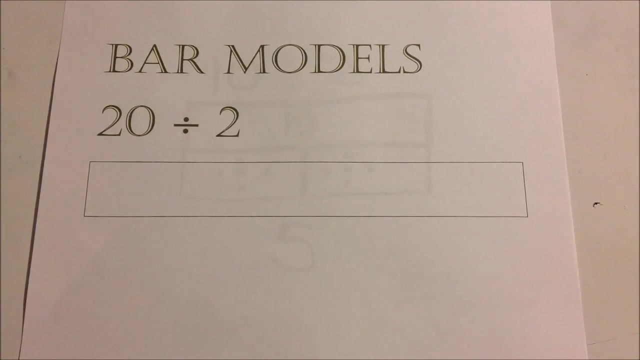 sign. and we know that there are five in each box. so we just model 10 divided by 2, and we know it equals 5. what if I gave you this? try that one. what goes in the box? well, the bar this is: we put a 20, good, and what are we? 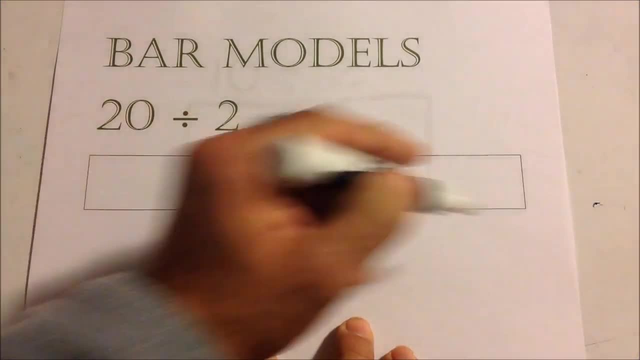 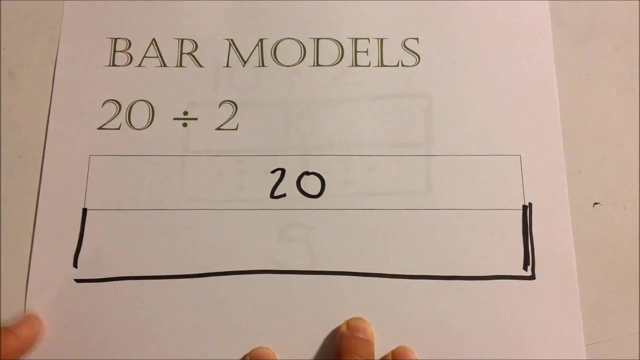 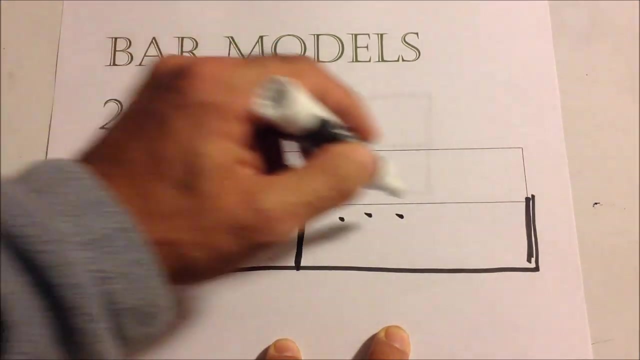 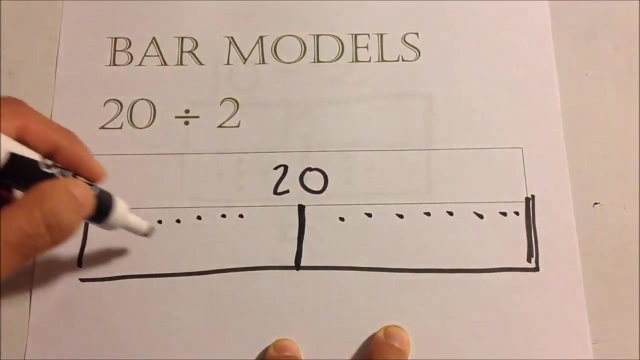 doing next step 2: make another bar. good, make another bar. and this is telling us to cut it twice right in half, And I know you can see that we should have 10 in each box, but we'll do it anyway. We'll go 1, 2,, 3,, 4,, 5,, 6,, 7,, 8,, 9,, 10,, 11,, 12,, 13,, 14,, 15,, 16,, 17,, 18,, 19, 20.. 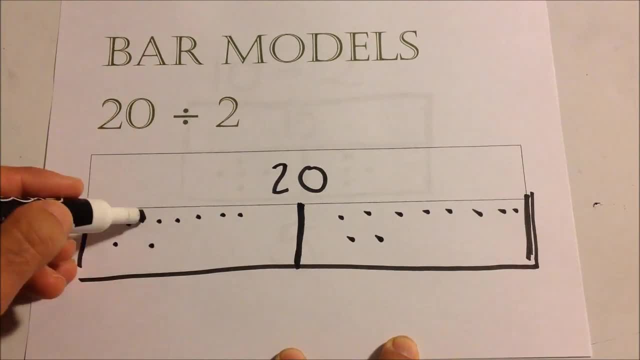 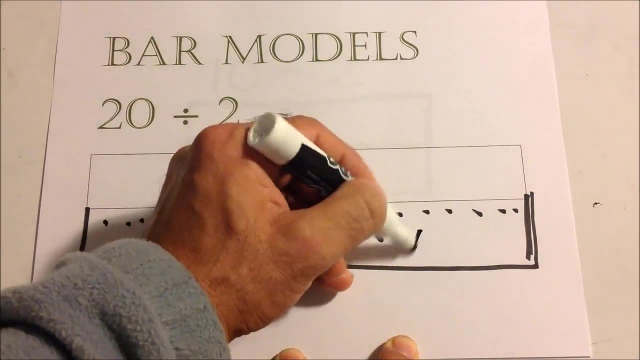 So we should have 10 dots: 1,, 2,, 3,, 4,, 5,, 6,, 7,, 8,, 9, 10.. 10 here, and 1,, 2,, 3,, 4,, 5,, 6,, 7,, 8,, 9,, 10.. 10 there. There's our bar model. 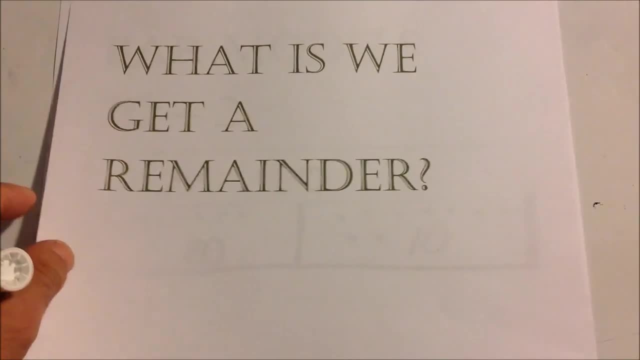 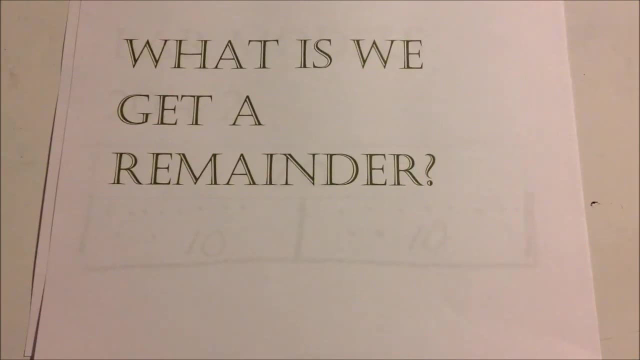 But wait a minute. What if we get a remainder? That pesky remainder, Remember? we kicked him out in 5th grade. So what if we had? Oh, we'll have a little earthquake there, Calm down. What if we had? 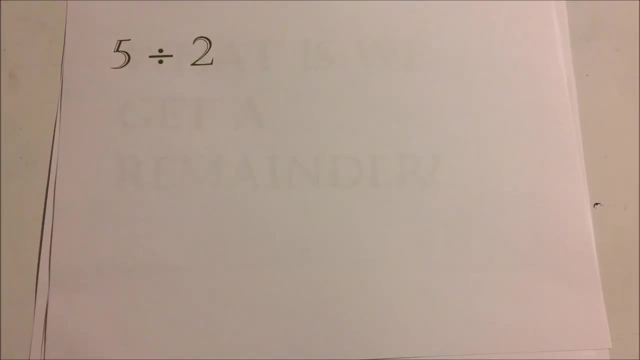 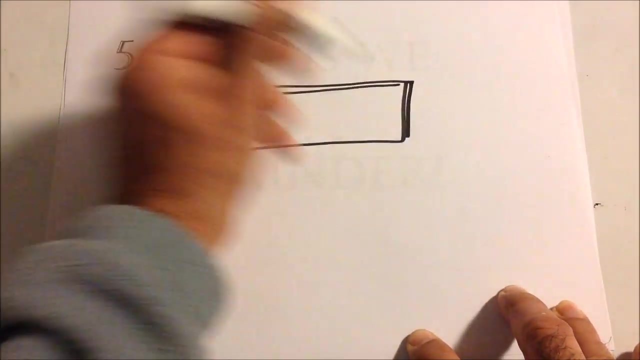 5 divided by 2.. So we'll do the same thing. We're going to make a bar, There's our bar, And we're going to put 5.. And we know we put another bar on the bottom. And how many times should I cut it? 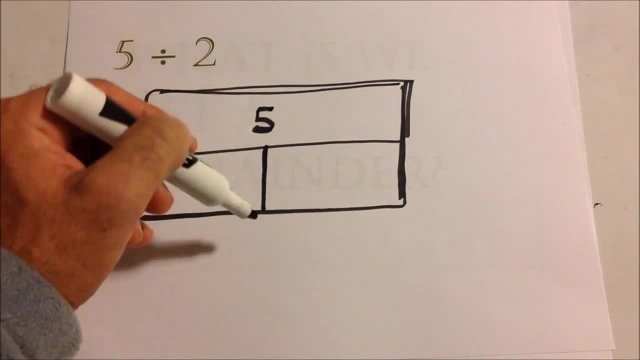 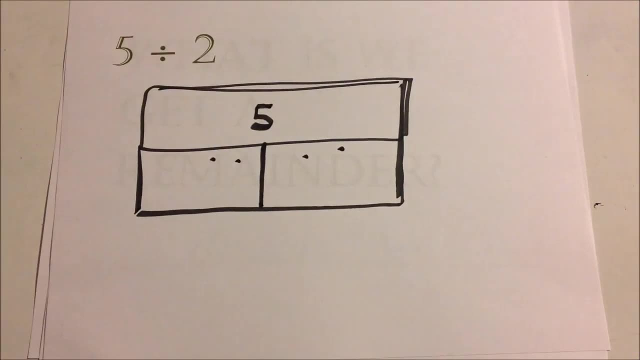 Twice, Because it says 2., 2 boxes. So now let's make 5.. 1,, 2,, 3,, 4.. We can only make 4.. We can only make 4. evenly, There's 1 remainder. 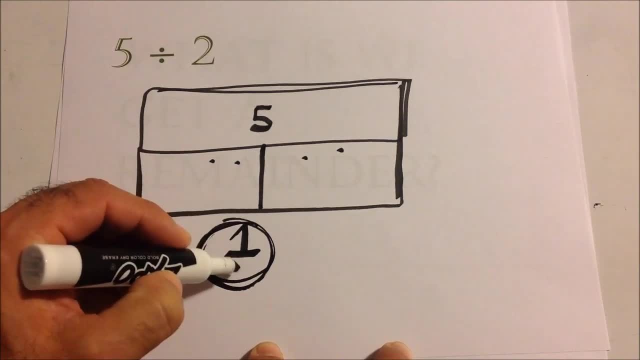 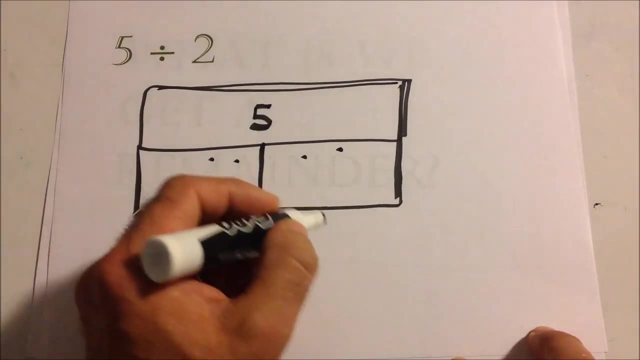 So what do we do with this remainder, This pesky remainder? So what you're going to do is you're going to take the remainder. This is what we're always going to do: We're going to take the remainder And we're going to make it a fraction. 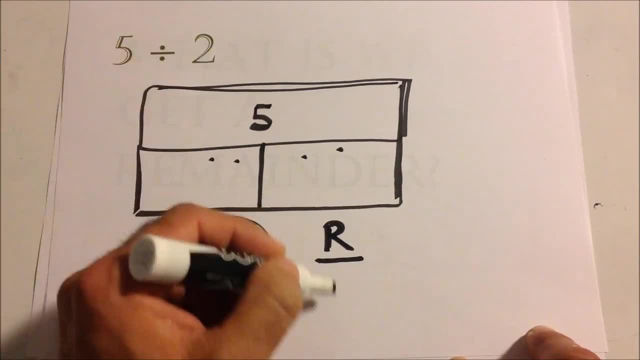 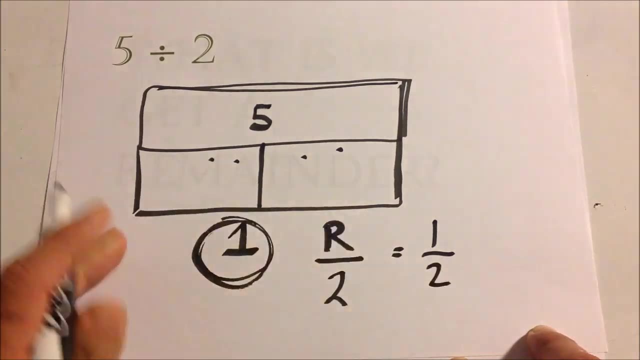 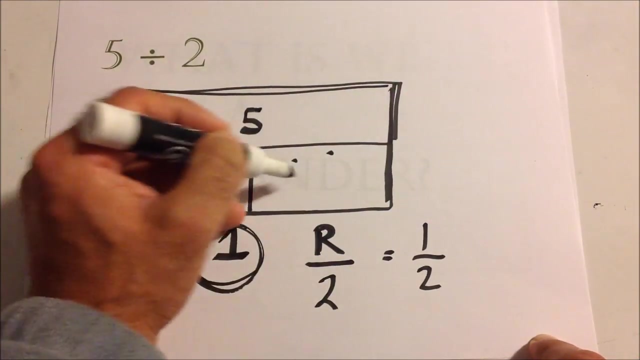 Put the remainder on top And the divisor on the bottom, So this remainder is 1.. So this will be 1 half. So our answer will be: we have 2. Right, 2 in each box. So we have 2 in each box. 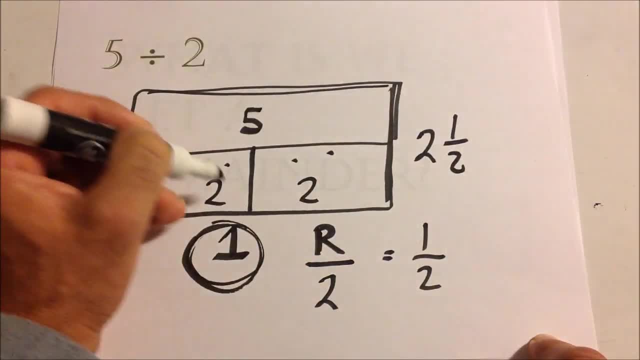 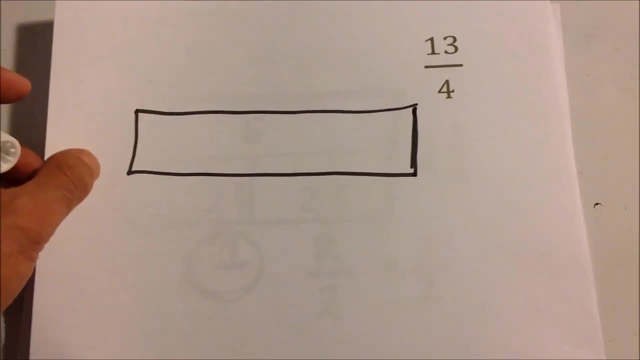 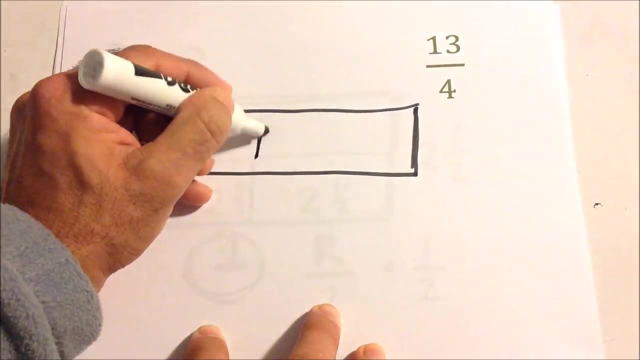 Our answer is 2 and a half. So that would be our bar model. I'll give you another example. Okay, what if we had this 13 divided by 4.. Remember, that's what it is. So here's our bar, And we're going to put a 13.. 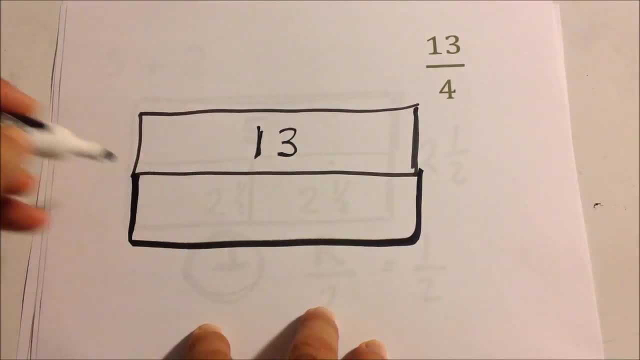 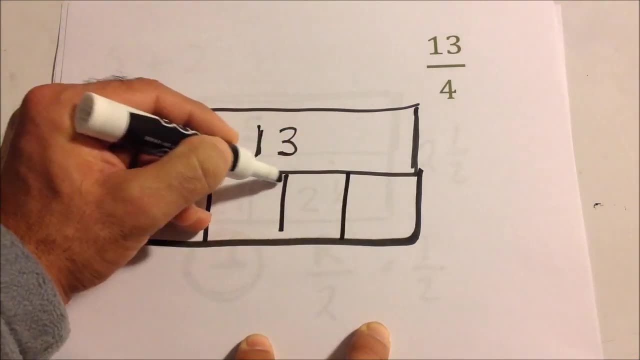 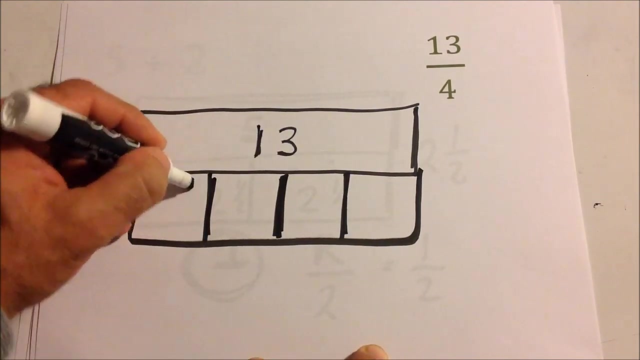 Step 1.. We make another bar, And what do we do with that? We have to cut it up 4 times. Okay, So now we have 4 times, We cut it up And let's do. now We'll put 1,, 2,, 3,, 4.. 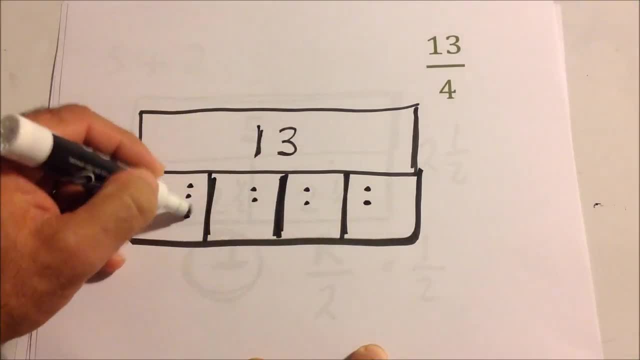 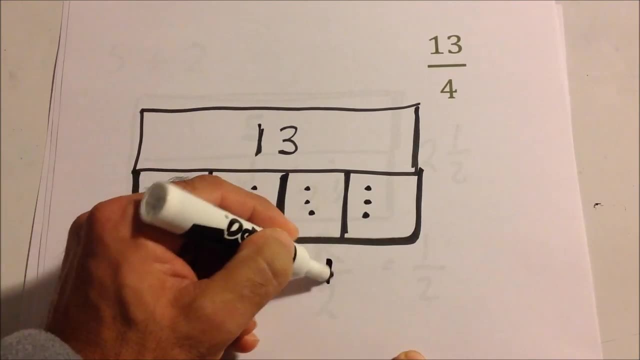 Everything has to be even: 5,, 6,, 7,, 8,, 9,, 10,, 11,, 12.. And guess what? We can't put them all in. There's 1 remainder, So it's 1 over 4.. 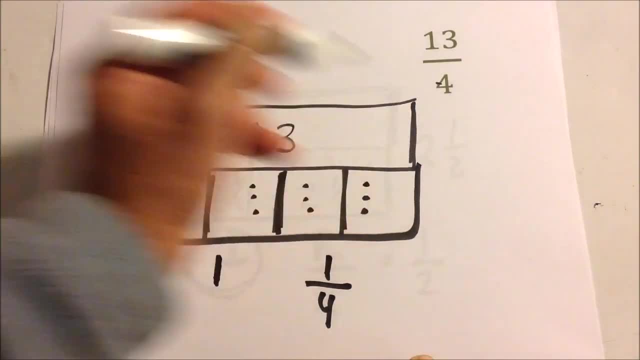 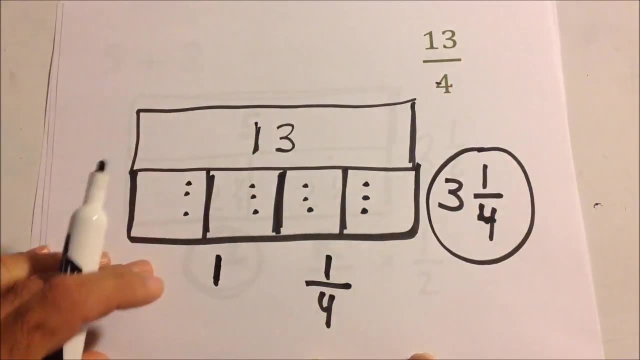 We put the divisor, We put the divisor on the bottom. So our answer is going to be: each box has 3.. So it's 3 and 1 fourth. That's our answer. So in other words, we have to take this 1.. 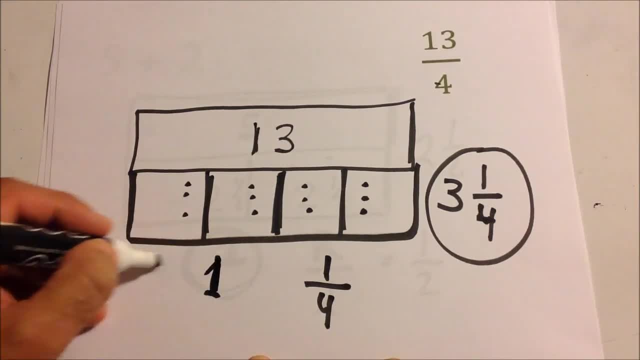 This 1 whole remainder And we have to cut it up 4 times Like a pizza. There it is 4 times, So each one's getting a fourth. You're getting a fourth in here, So this will be 3 and a fourth. 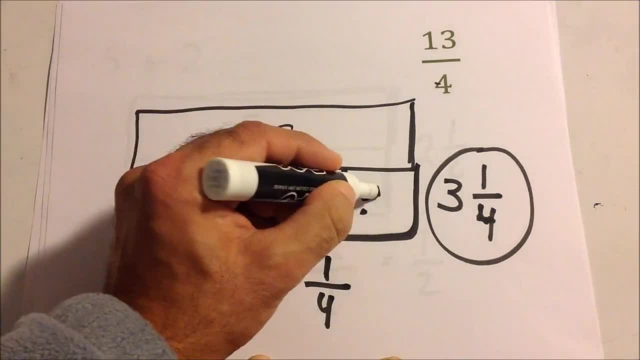 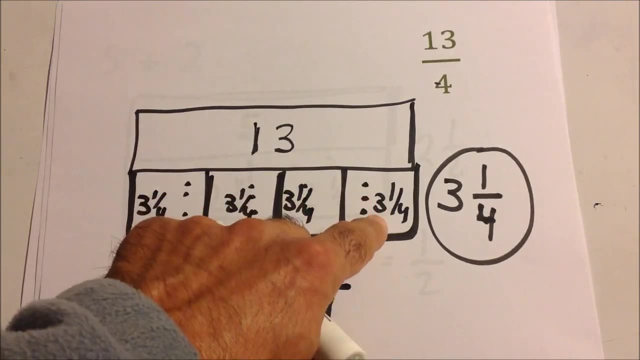 3 and a fourth, 3 and 1 fourth And 3 and 1 fourth, So we have 3,, 6,, 9,, 10,, 11,, 12.. And those 4 fourths- 1,, 2,, 3, 4- make 1 whole number. 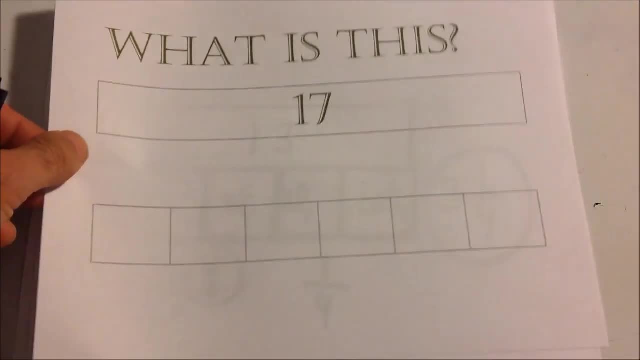 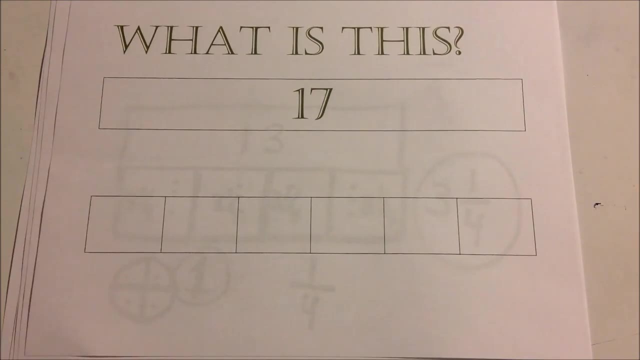 That's why we have 3 and 1. fourth, What if I gave you this? I gave you this model. What division problem is this? What do you think? I'll give you a few seconds. Well, we know, The top number tells us it's the dividend. 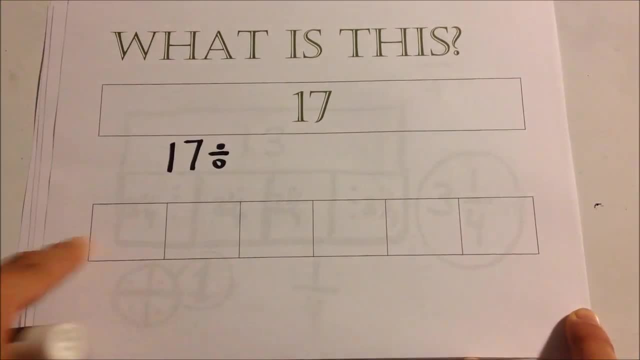 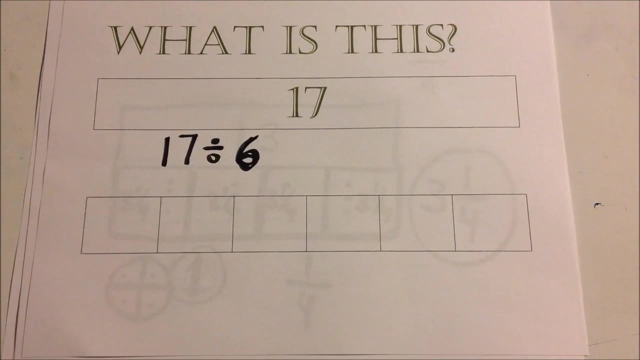 It's 17 divided by, And the boxes tell you what we're dividing by: 1,, 2,, 3,, 4,, 5, 6.. 17 divided by 6.. There it is, Let's do. 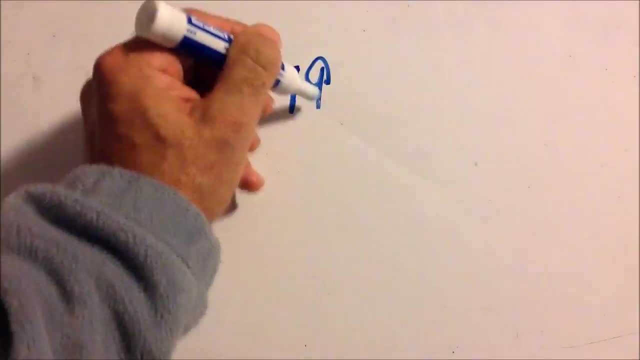 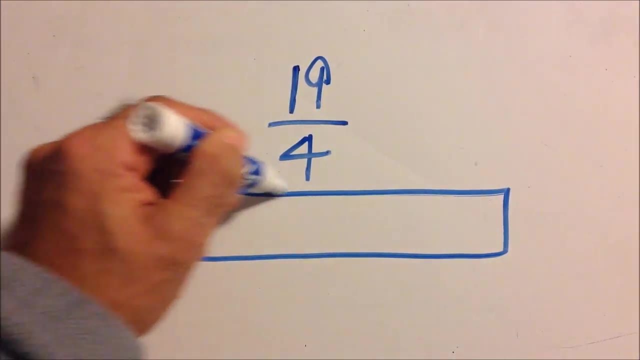 What if we did? Let's do 19 divided by 4.. Use 4 again. Okay, What's the first step? Make a bar. Here's our bar, And 19 goes in the middle. You knew that right. 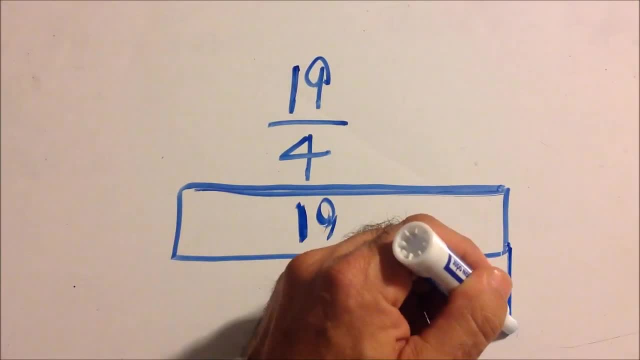 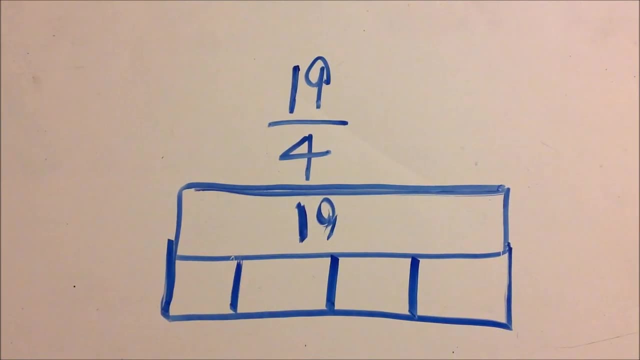 Well, that doesn't look like the middle, but it's there. And then what's the next step? Make another bar, That's right. Cut it up 4 times, That's right, Okay. So let's use a different color.